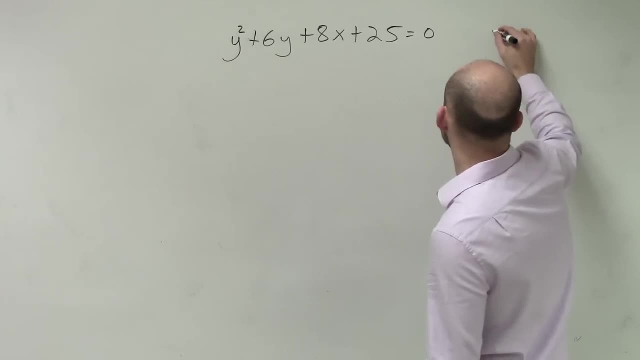 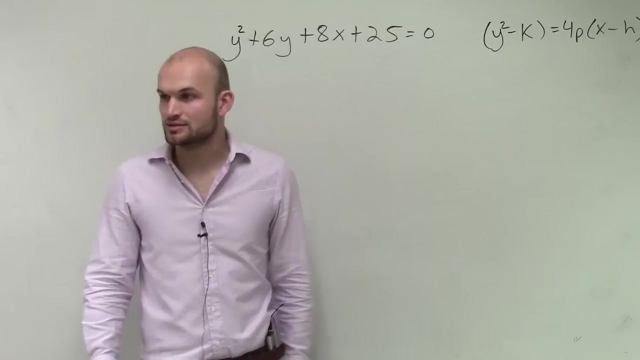 of our parabola when our Y is squared. So we say Y squared minus K equals 4P, X minus H. Alright, I did find my formula sheet so you guys won't have to worry about all this stuff, But you guys need to get these formulas Understand, right, Okay? So now we need to. 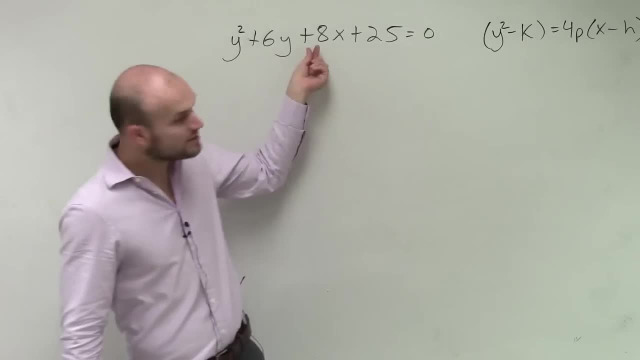 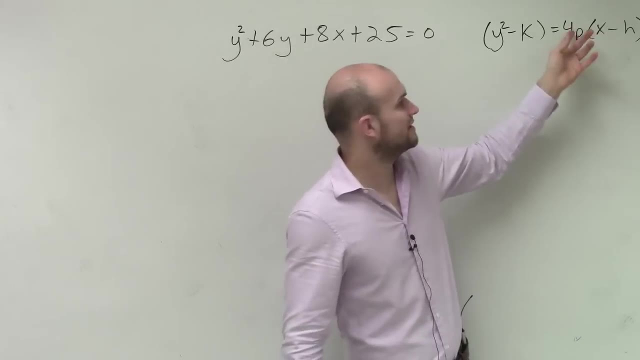 make this look like that, Because once we know that, once this looks like that, is it pretty easy to find the vertex director, except the focus. Yeah, the vertex is there, then you know P, then you can find focus director. so it's easy. Yes, it is, I don't. 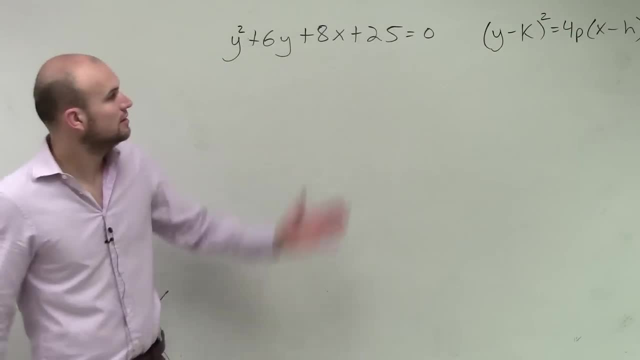 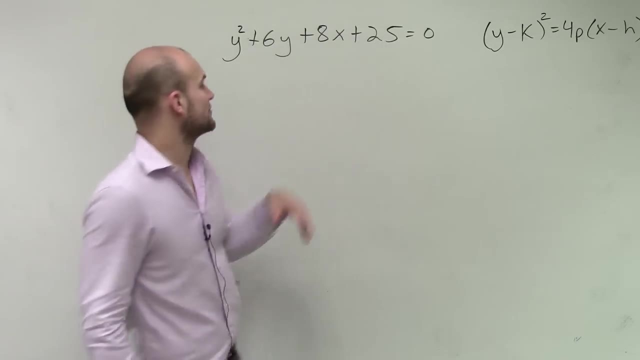 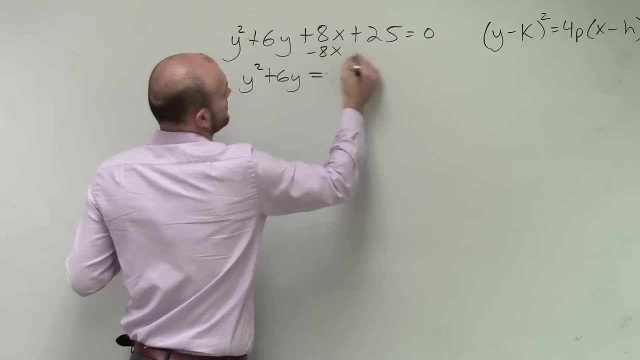 know why. Thank you, Okay. So to make this look like this, let's get the X's on the other side right, And this: let's get the X's over here. So I have Y squared plus 6Y equals minus. 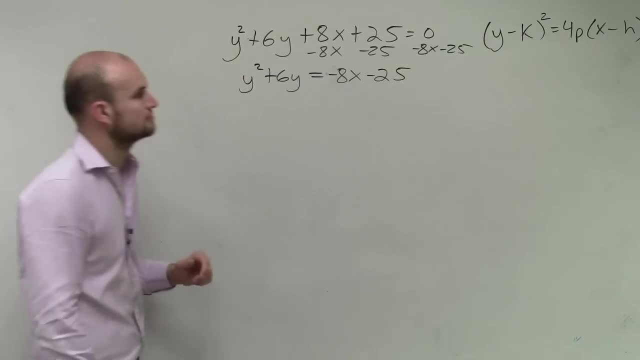 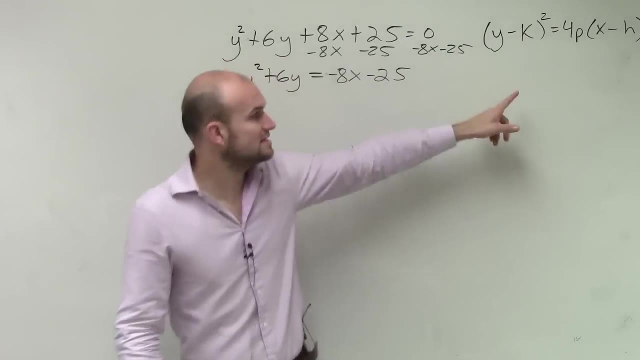 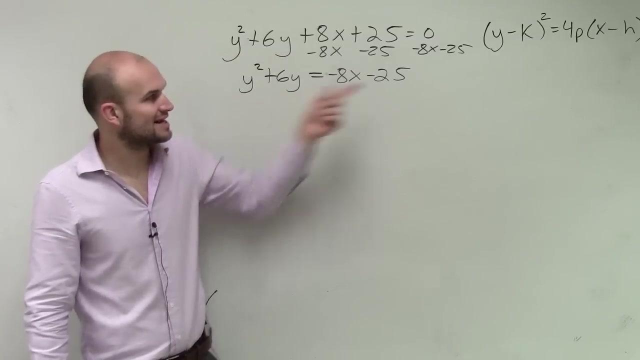 8X minus 25.. Alright, This looks kinda like there, but you can see that this is a binomial square, right? And this is not a binomial square, So you could factor out a Y, but that's not gonna. 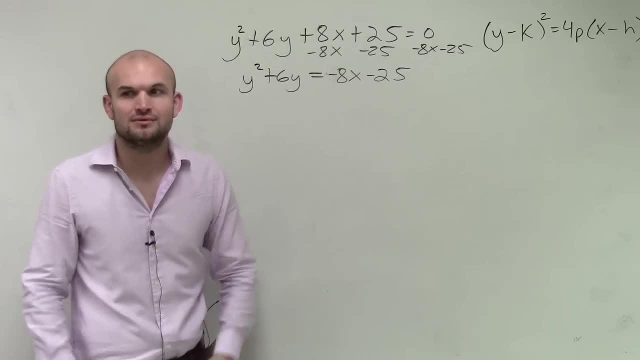 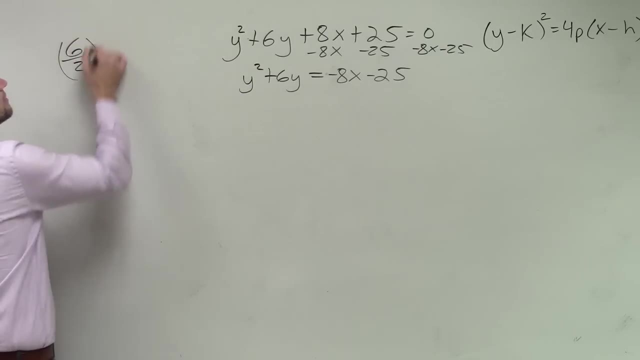 make it look like that. So to make this a binomial square, we have to complete the square right. So if you guys remember completing the square, you take your B 6, divided by 2, square it, which equals. 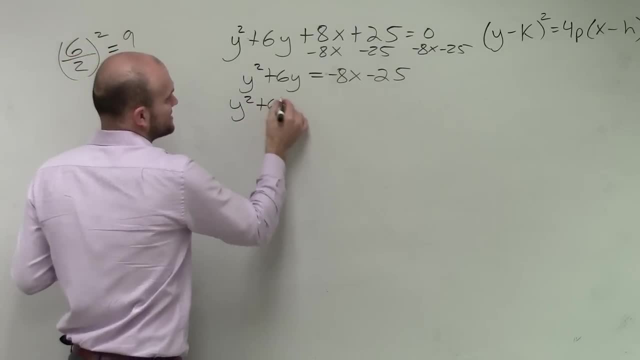 9. Then we add 9 on both sides, Y squared plus 6Y, and I'll even use a little comma and I'll make it 하고 two. So this is how we're gonna do it. I'm just gonna jump right. 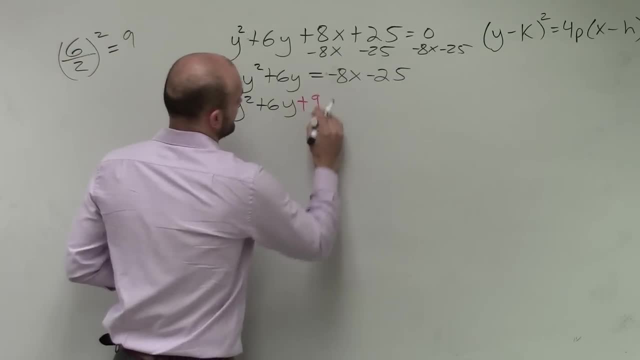 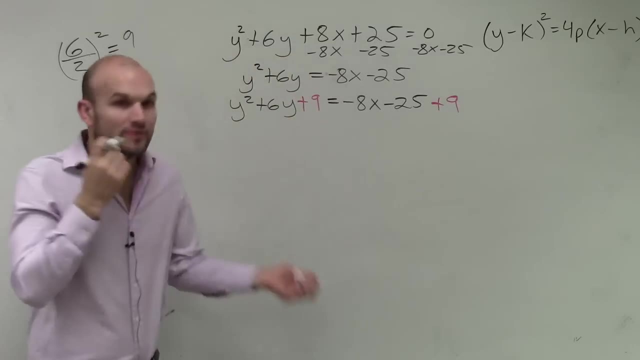 I'm going to use a little color. plus 9 equals negative 8x minus 25 plus 9.. And why do we complete the square? The reason why we want to complete the square is because when we take b divided by 2 and square it, 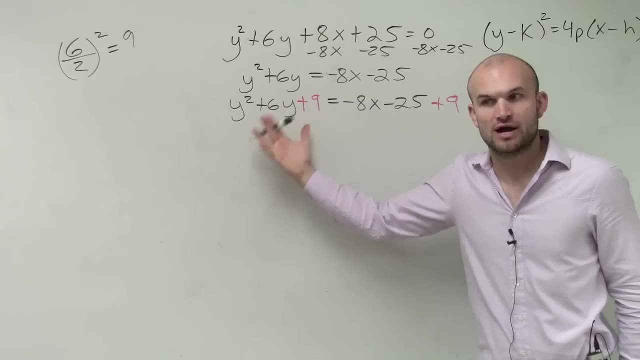 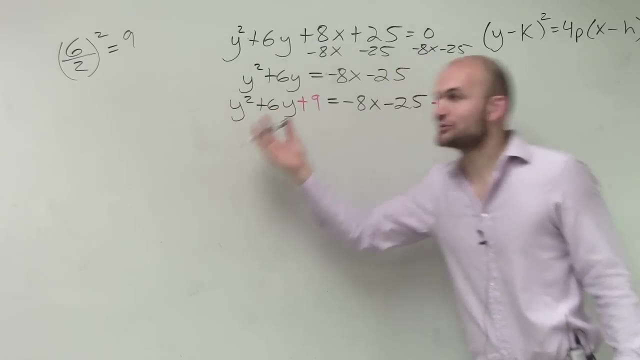 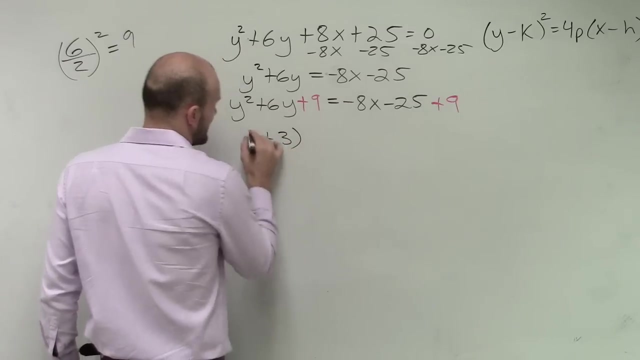 we now have just created a perfect square trinomial. And why is perfect square trinomial so nice? Because perfect square trinomials can be factored to a binomial square, And in this case we can rewrite this as y plus 3 squared. 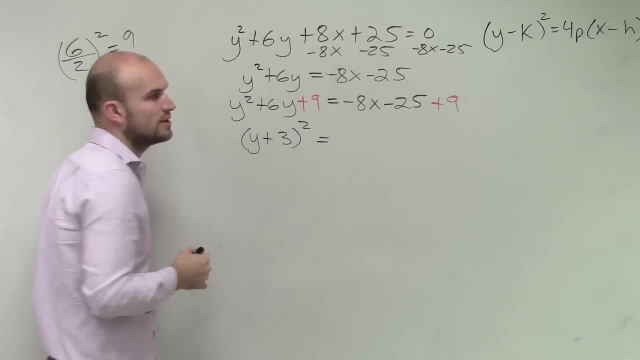 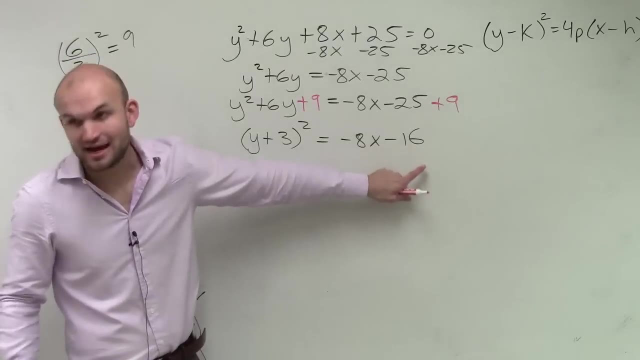 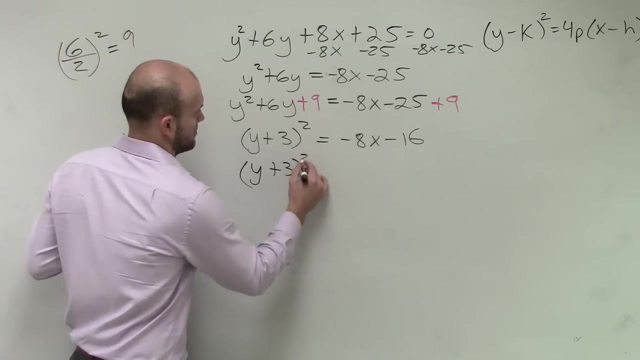 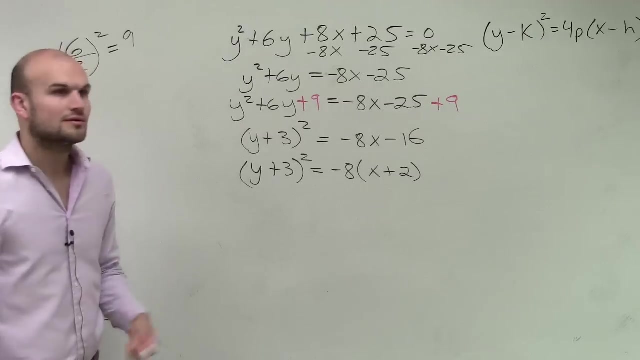 Then we just do a little simple math over here. Negative 25 plus 9 is going to give me a negative 16,. right, And now I can factor out a. I can factor out a negative 8.. Now does it look like it's in our formula? 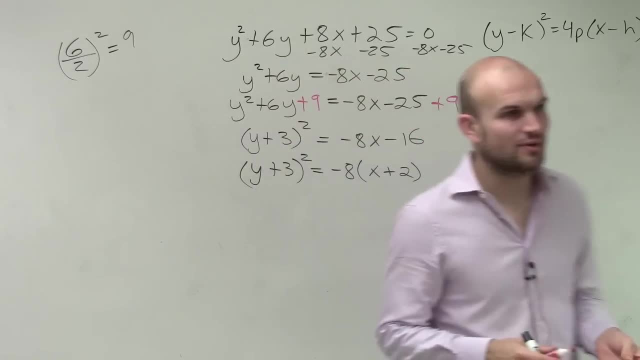 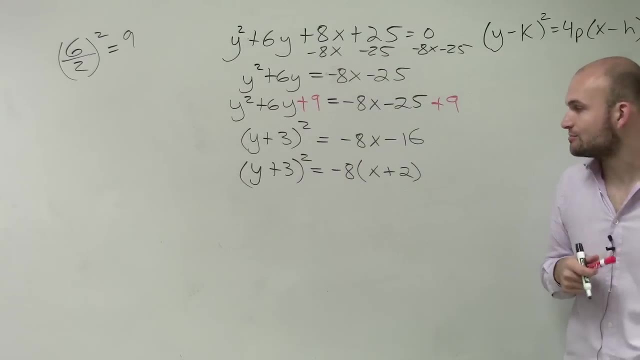 Yeah, absolutely So. do you guys see how just completing the square is just going to help us apply that? So if you don't have it as a binomial square, you're going to have to complete, you're going to have to use the process of completing the square. 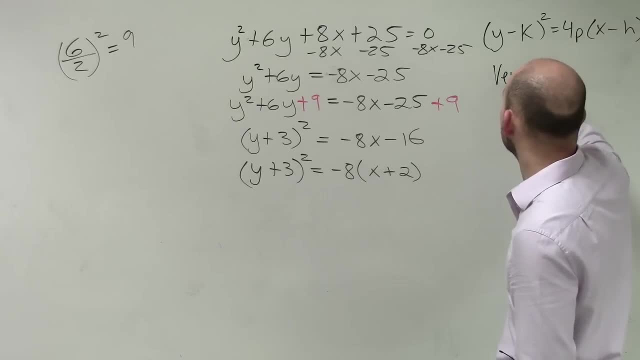 All right, so now let's just go through it. So the vertex, we know is hk. Remember it's opposite of k, opposite of h. And then also, ladies and gentlemen, remember that here's the k and here's the h. right. 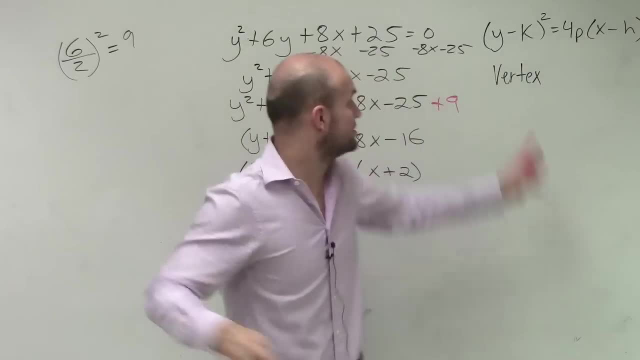 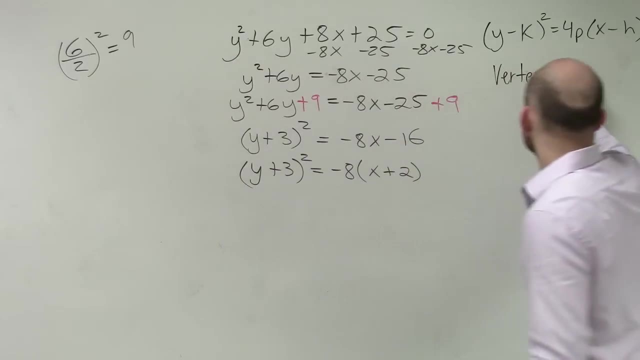 A lot of students because they know that for vertical parabolas it was h and k, All right. so they say, oh, the vertex is going to be negative, 3, negative, 2.. Be careful, Here's your h, and so your vertex in this case is negative, 2, negative, 3.. 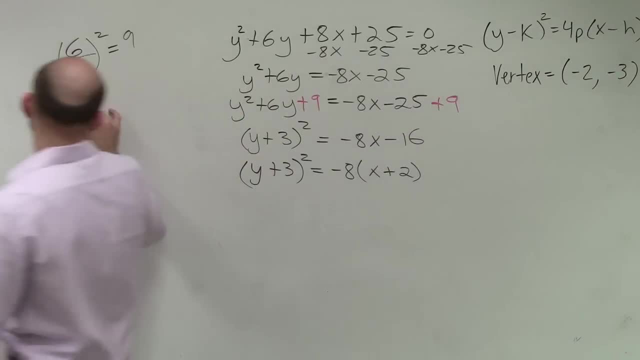 Now what does our 4p equal? 4p equals negative 8. So we say: negative 8 equals 4p divided by 4, divided by 4p equals negative 2. So now we know p is negative 2.. 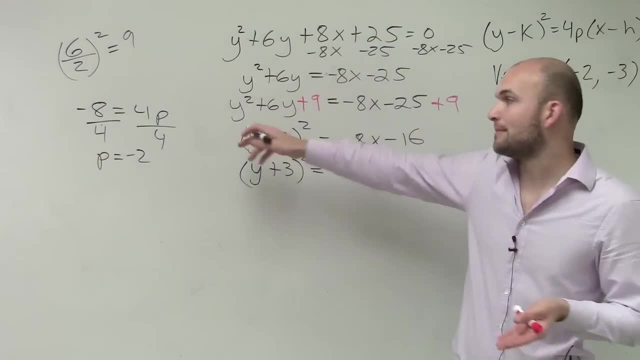 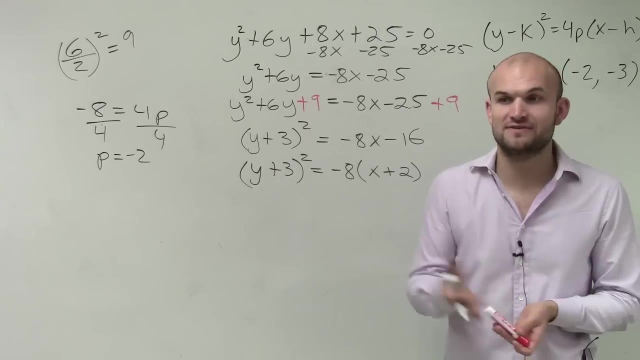 Does that mean, since my graph opens right or left. when my p is to the left, that means my graph is now going to open Or, I'm sorry, p is negative, so that means my graph is not going to open to the left right? 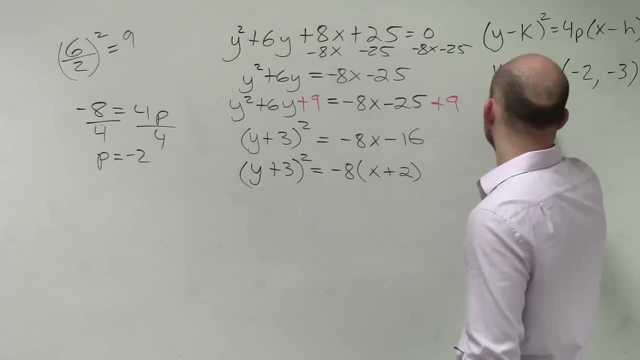 So, again, to find the focus, since we're shifting left and right, we're not going up and down, remember, we're going to be adding points to the remember vertex, or it's h, k, So the focus is going to be h plus p k. 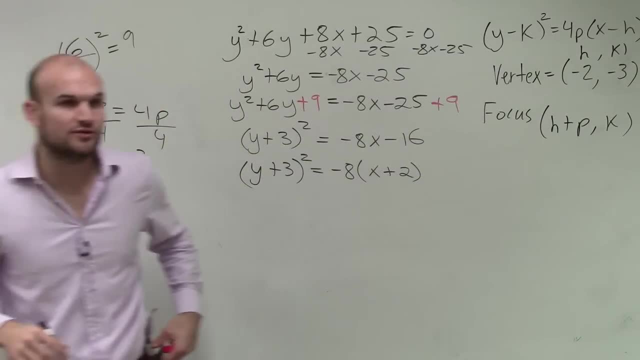 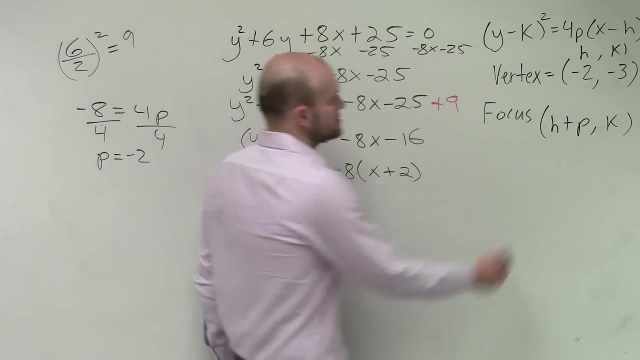 Notice how that's different than what it was for the vertical parabola. The vertical parabola It was plus k, Now it's going to be plus h, because h is your x coordinate. So we look at this and we say negative 2 plus negative 2 comma, negative 3..